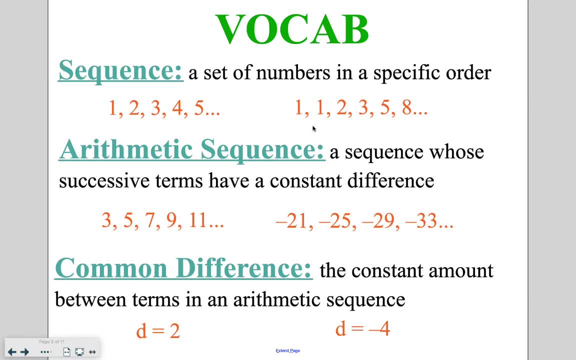 order. We're going up by one every time. This next set is also a sequence. So we start with one, we add zero to get to one, we add one to get to two, we add one to get to three, then we add two, 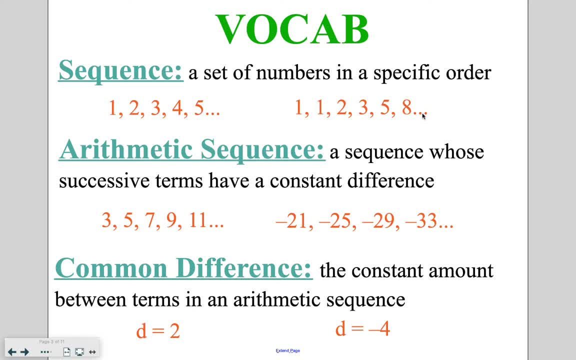 then we add three, then we would add five, then we would add eight. This particular sequence is called a sequence of numbers. So we're going to start with one, we add zero to get to one, 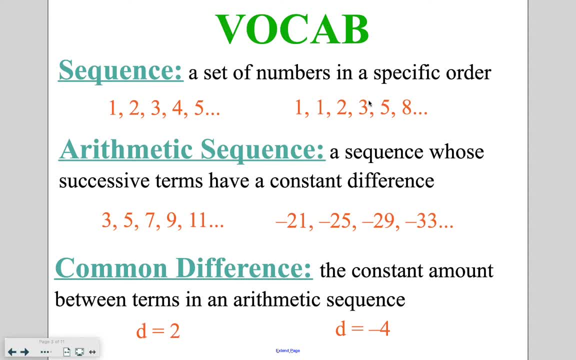 the Fibonacci sequence. It is not an example of an arithmetic sequence. An arithmetic sequence is a sequence whose successive terms have a constant difference. So what that means is we get from one number to the next number by adding. When it's talking about terms, it's talking about 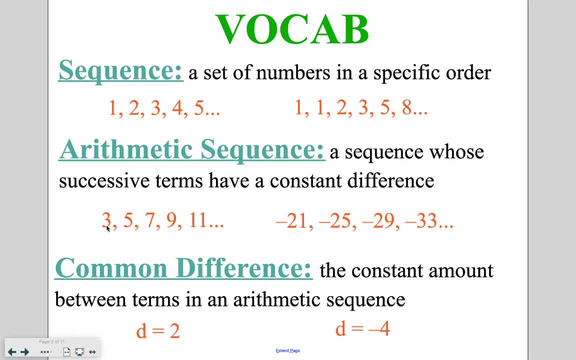 the numbers in order. So in this example, three is the first term, five is the second term, seven is the third term. We get, to each term in this sequence by adding two. In the next example over here, we get to every number 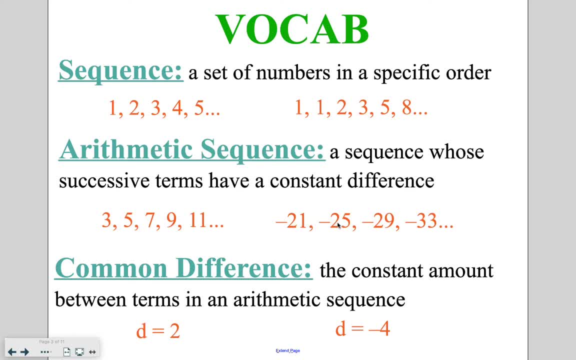 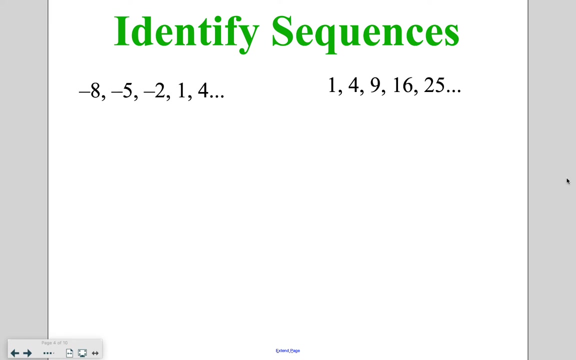 by subtracting four. Those values that you are adding or subtracting by is called the common difference. So we would write that out for this three, five, seven, nine, 11 sequence. We would say D, which stands for the difference, is equal to two. For the negative 21, negative 25, negative 29, negative 33, we would say D is equal to negative four because we are subtracting by four in between every term. So our first job is to identify whether a sequence is arithmetic or not. 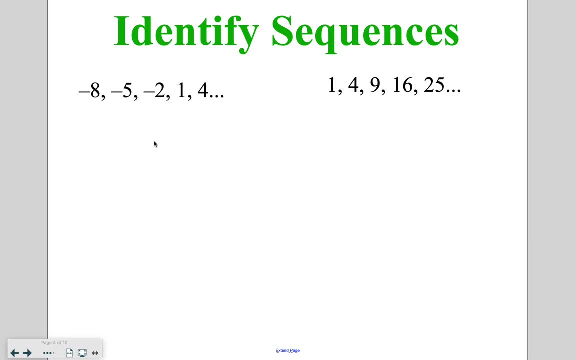 Again, we're going to do this by looking for a common difference. So we're going to look at our sequence and I've got negative eight to negative five. That is a difference of plus three. Negative five to negative two, once again, difference of plus three. Negative two to positive one, once again, plus three. And one to four is plus three. So this is an arithmetic sequence. And your reason would be common difference is equal to three. So we give 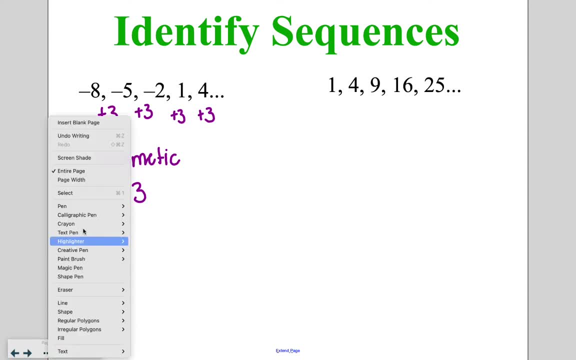 the value that we are increasing by. If I look over at my next sequence, I've got one to four is plus five. Four to nine is plus five. Nine to 16 is plus seven. So we can already tell this is not 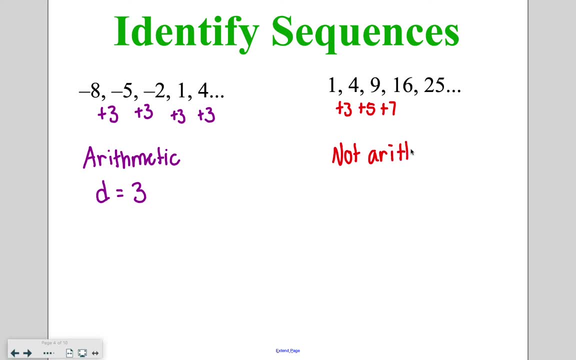 arithmetic. You actually could have discovered that after the first two. And that is because there is no common difference. So if it is not an arithmetic sequence, we need to write out the fact that there is no common difference. That is what makes it non-arithmetic. Go ahead and try this 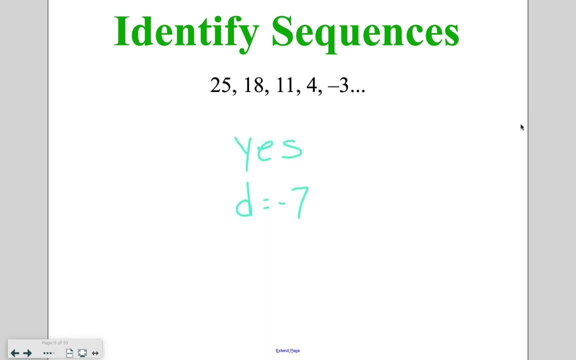 one on your own. In this case, your sequence is arithmetic and you are subtracting by a common 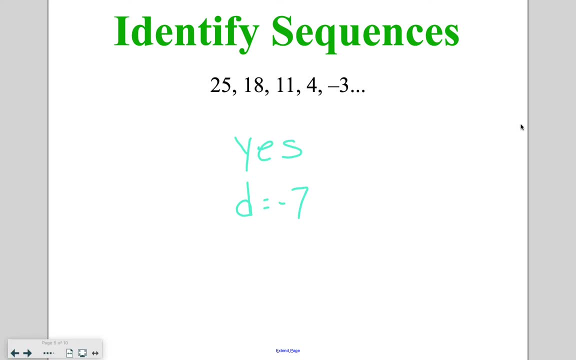 difference of seven every time. So once we have a sequence, the next thing we can do is add on to it. So going back to that example from the first one, 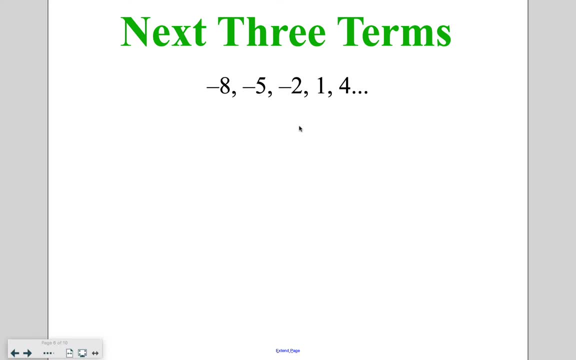 where I had negative eight, negative five, negative two, positive one, positive four, my common difference was adding three. So my next term then after four would be four plus three, which would give me seven. Then I would do seven plus three, which would give me ten. And then I do ten plus three, which would give me thirteen. So my next three terms would be seven, ten, and thirteen. 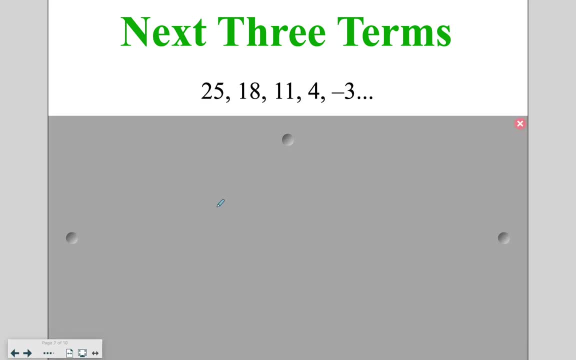 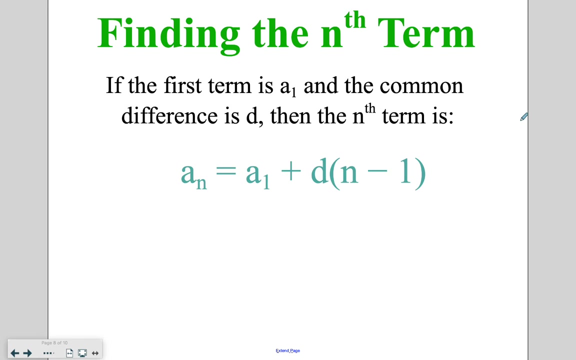 Go ahead and find the next three terms for this sequence on your own. Subtracting our seven, we get negative ten, negative seventeen, and negative twenty-four. Sometimes we want to be able to move beyond just the next three, or four, or five terms and we want to find something much further along in the sequence. In order to do that, we can use the equation seen here. 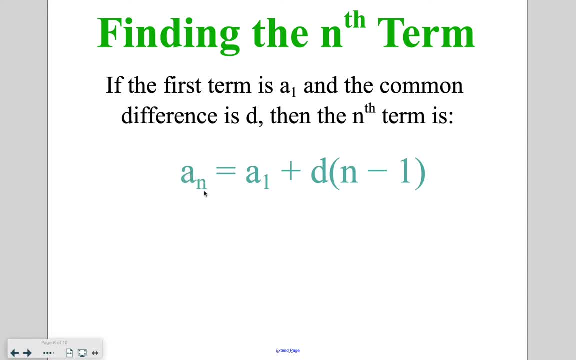 This A-N stands for A-any number, so any number within the sequence. 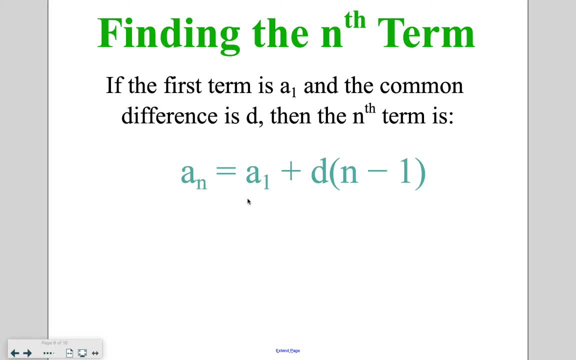 The first term is represented by A-1, so this is the first number listed in your sequence. 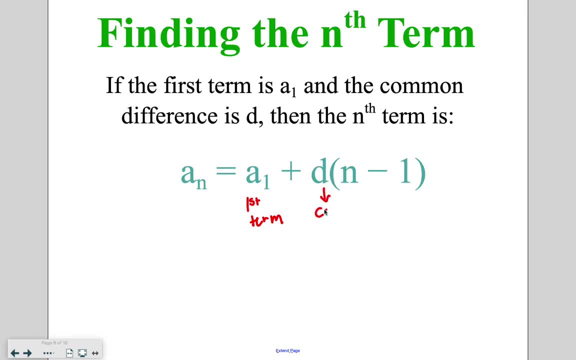 The D stands for that common difference that we were talking about, so how we get from number to number. 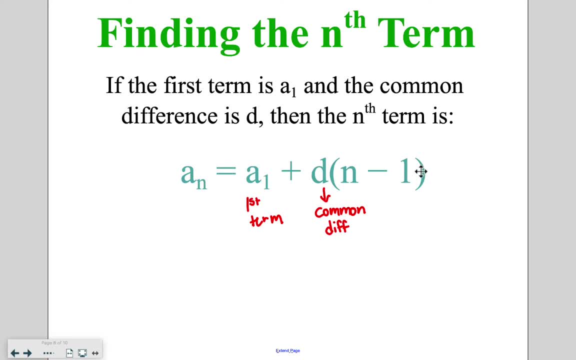 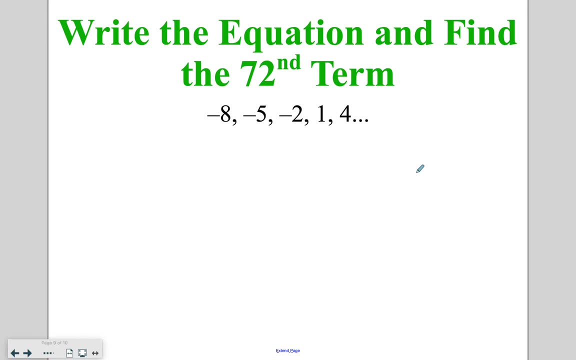 And then we have N-1 in parentheses as part of our expression. So, if I'm looking at the sequence that I've been looking at, negative 8, negative 5, negative 2, 1, and 4, 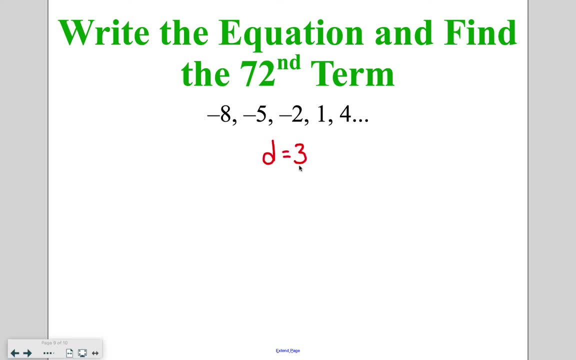 my common difference is still 3, and my A-1 term is negative 8. So when I start writing this expression, I would say A-N, 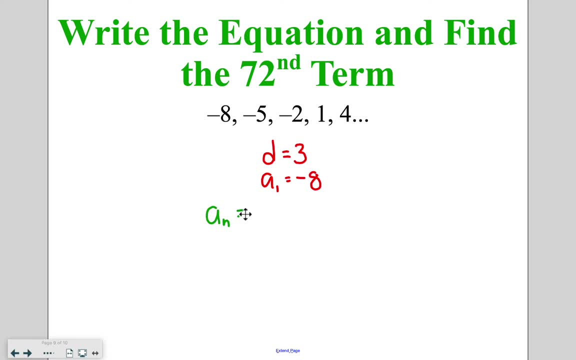 notice that N is in the subscript, and that's going to equal my A-1 term, which is negative 8, plus 3, because my common difference was positive 3, and then in parentheses, N-1. So that's how I start my equation. I now need to simplify it. 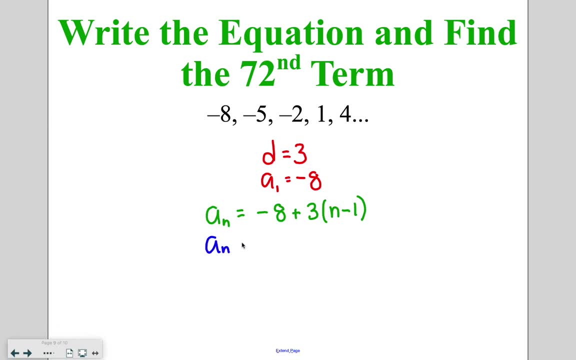 The first thing I'm going to get rid of is those parentheses. So I've got A-N is equal to negative 8, 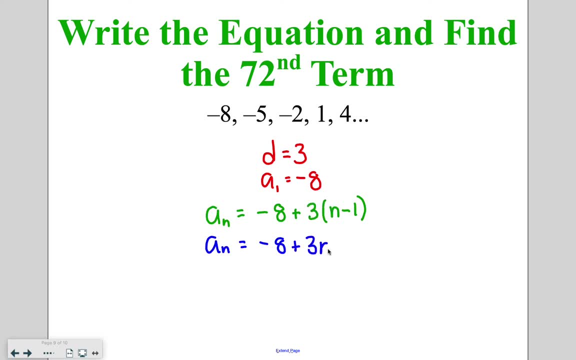 plus 3 times N, which is 3N, and then 3 times negative 1, which is negative 3. 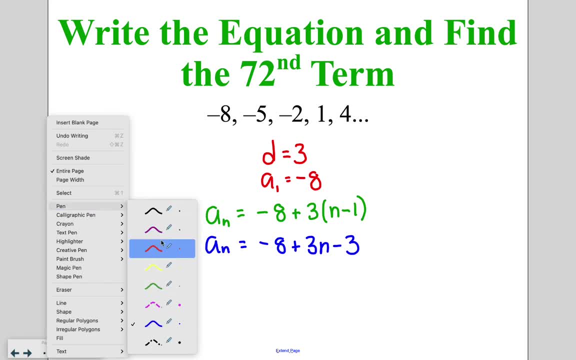 So I've gotten rid of my parentheses, and now I need to combine my like terms. 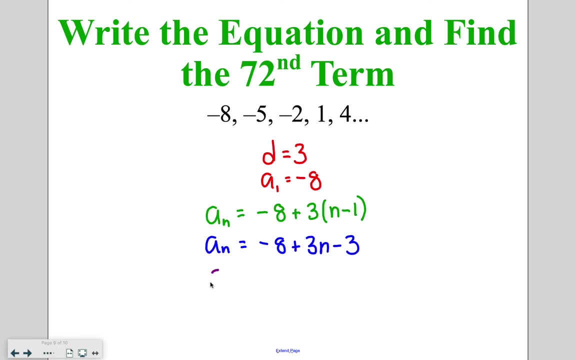 Negative 8 can go with negative 3, so I end up with A-N is equal to the 3Ns, and then negative 8 minus 3 gives me negative 11. 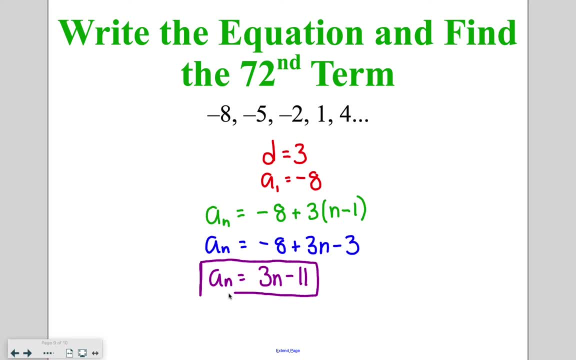 So my equation that I'm going to use for this sequence is A-N is equal to 3N. That's the writing the equation part. 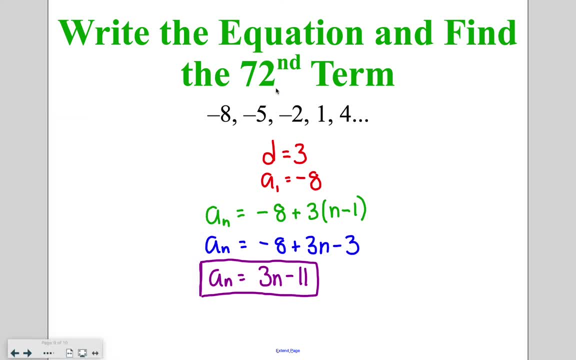 The other piece that it asks us for is to find the 72nd term. 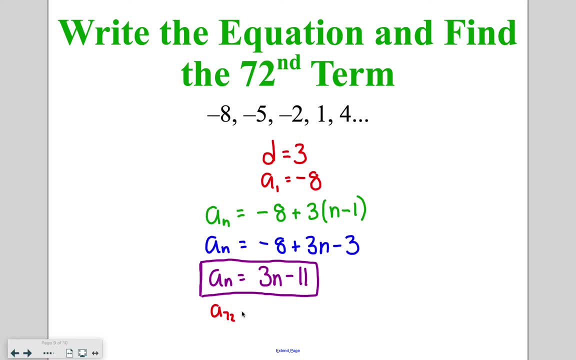 So when I do that, I'm going to say A-72 is equal to 3 times 72 minus 11. 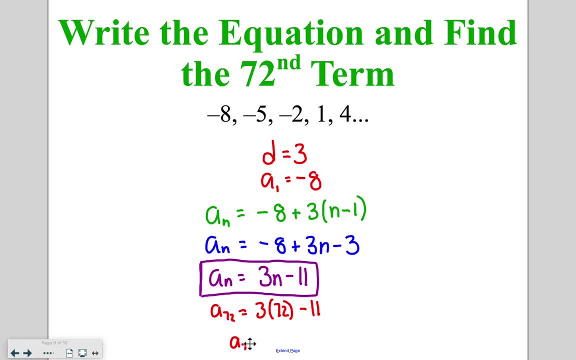 So what I would write as my answer then is I would say A-72, so saying the 72nd number in the order, is equal to 3N.